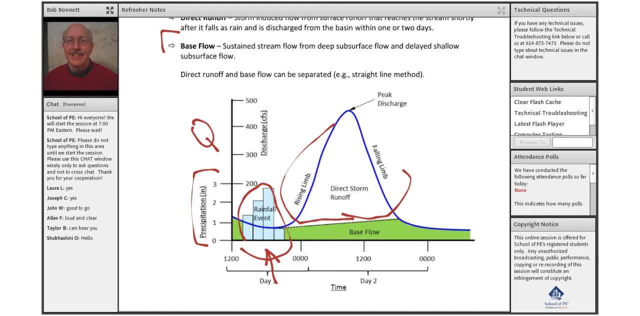 then is going to increase the level in the stream as flow goes into the stream And there's going to be a lag between the rainfall event and what's going to be the peak of your hydrograph. And there's other terms like the level in the stream is rising, rising limb of the hydrograph and falling limb. 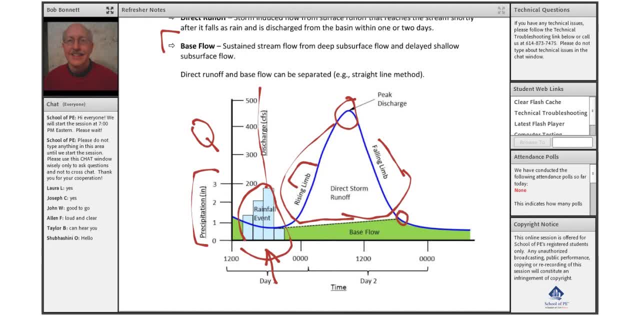 And then it comes back to base flow. After all that rainfall event, precipitation has completed its runoff and the stage or level in the stream or river have come back to normal or base flow. Notice the time duration can be as many as units of days or many hours. 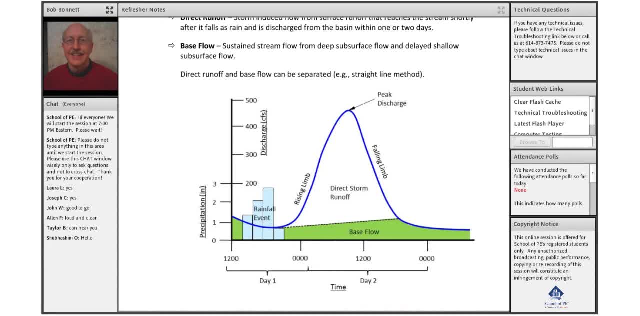 Okay, So there's two pieces of data. Okay, So there's two pieces of data. So there's two pieces of data. Okay, So there's two pieces of data. This is the data plotted there: rainfall event and what's your flow rate in your stream. 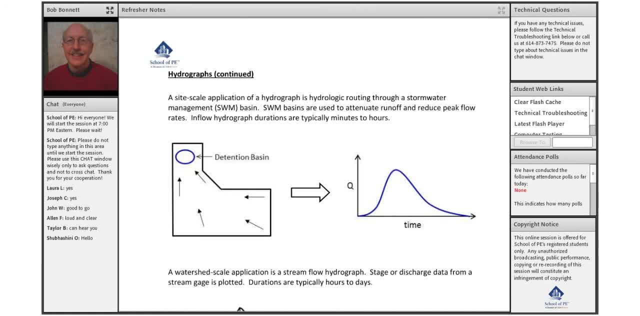 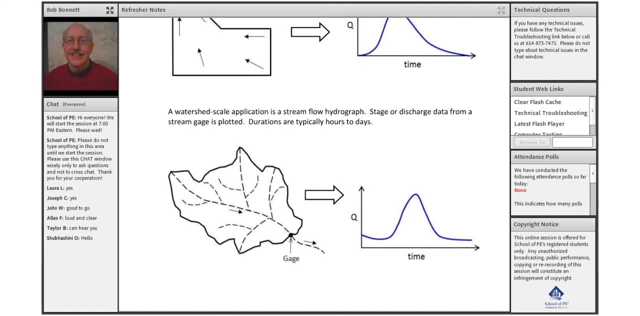 Moving on to the next page, as a refresher, hydrographs not only can be for what we see at the bottom figure of this page 66, where it is a drainage basin area in plan view with a lot of tributaries coming into and a gauging station. 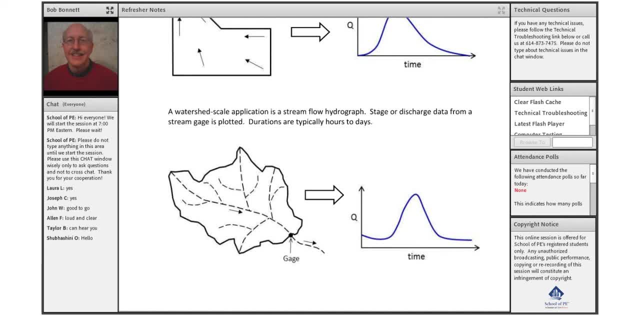 Let's start with that one first, And it's going to then have a hydrograph that looks like this on the right. it has a base flow, primarily from the groundwater, and then it has what from the precipitation that falls on the drainage basin area or watershed. it's 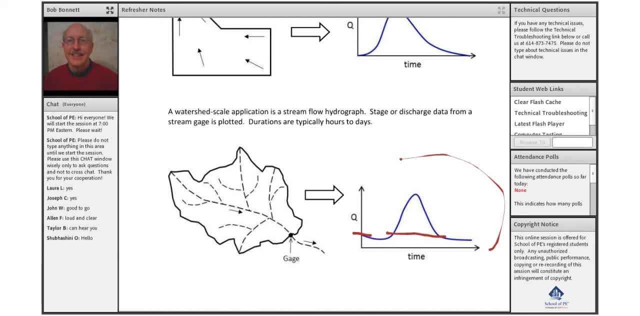 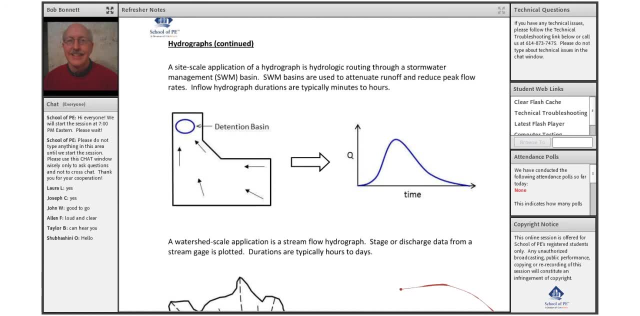 going to have this rise and that's come back down for the reasons that we stated. figures at the top hydrographs can be plotted for, say, a parking lot area. you can see that the flow is coming off and grade is sloped towards a detention basin in this particular hydrograph. that's on the right. it starts here at. 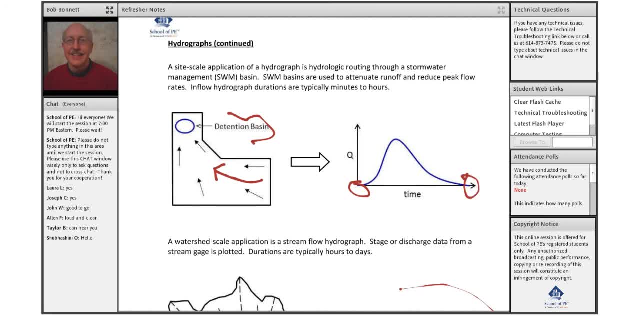 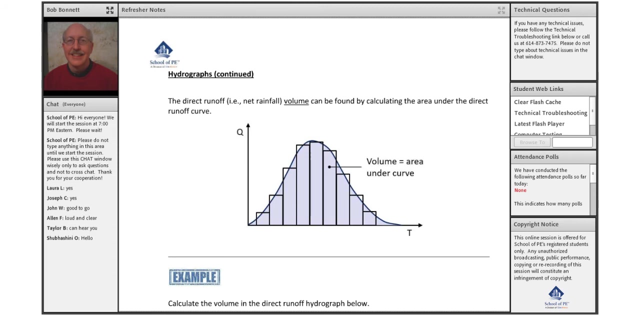 the ordinate and it ends at the ordinate because there isn't any extra level and on that pavement it's going to completely, you know, drain off into the detention basin. okay, alright, moving on to the next page part of this hydrograph separation method. if we've removed the base flow, we now have what's left is the direct runoff or net.